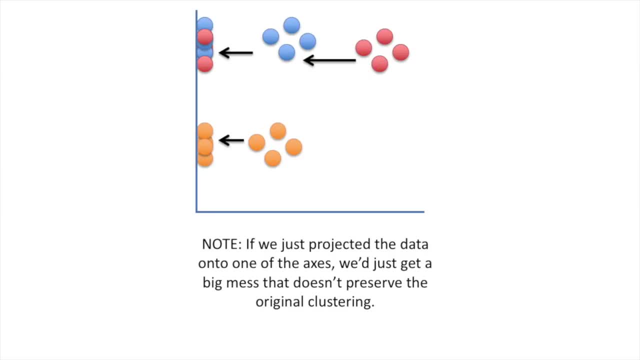 if we just projected the data onto one of the axes, we just get a big mess that doesn't preserve the original clustering. If we take a smaller data set and put it on the bottom of the graph, we get the same outcome. Let's try that again. 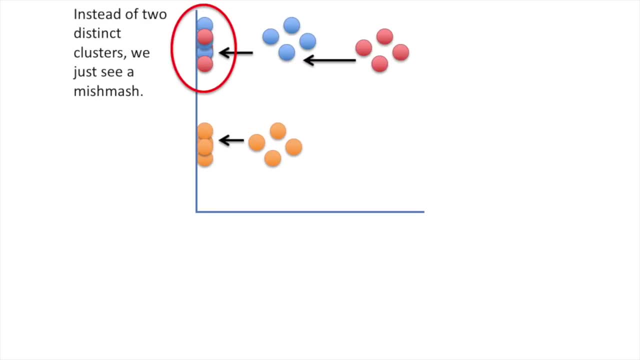 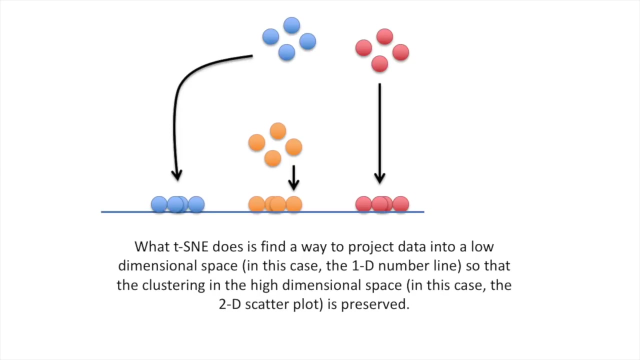 If we project it onto the y-axis instead of two distinct clusters, we just see a mish-mash. And the same thing happens if we just project the data onto the x-axis. What t-SNE does is find a way to project data into a low-dimensional space. in this case, 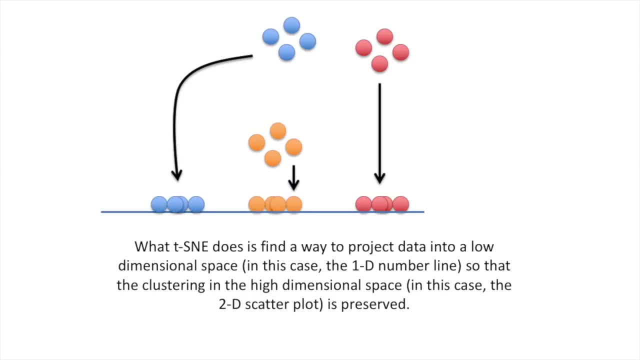 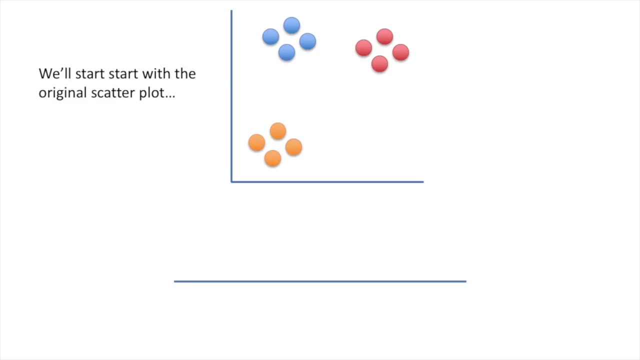 the one-dimensional number line, so that the clustering in the high-dimensional space, in this case the two-dimensional scatter plot, is preserved. So let's step through the basic ideas of how t-SNE does this. We'll start with the original scatter plot. 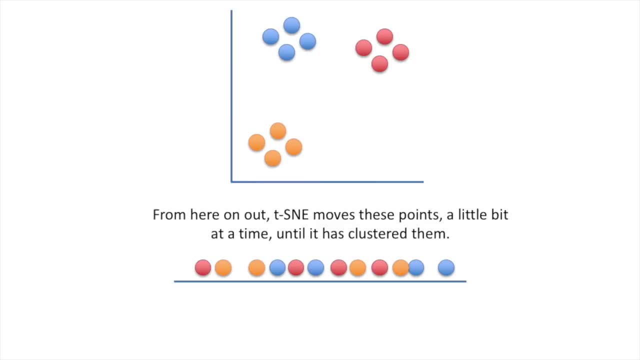 Then we'll put the points on the number line in a random order. From here on out, t-SNE moves these points a little bit at a time until it has clustered them. Let's figure out where to move this first point. Should it move a little to the left or a little to the right? 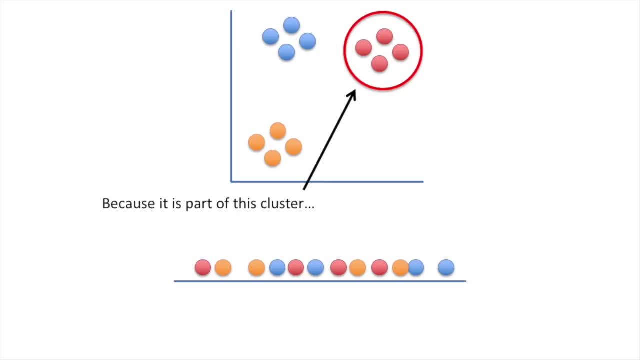 Because it is part of this cluster in the two-dimensional scatter plot. it wants to move closer to these points, But at the same time these points are far away in the scatter plot, so they push back. These points attract, while these points repel. 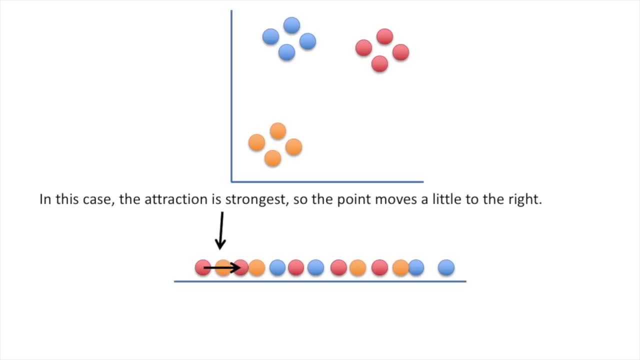 In this case the attraction is strongest, so the point moves a little to the right. Bam. Now let's move this point a little bit. These points attract because they are close to each other in the two-dimensional scatter plot And this point repels a little bit because it is far from the point in the two-dimensional 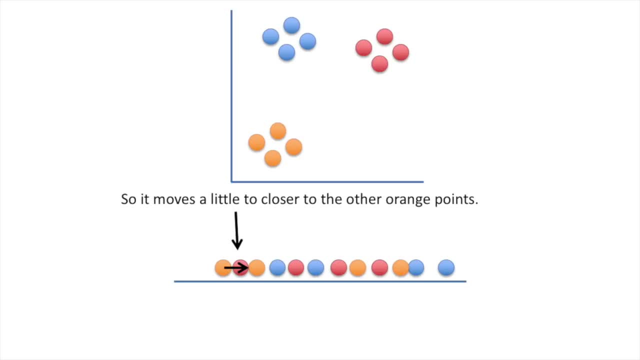 scatter plot. So it moves a little closer to the other orange points, Double bam. At each step a point on the line is attracted to points. it is near in the scatter plot and repelled by points. it is far from Triple bam. 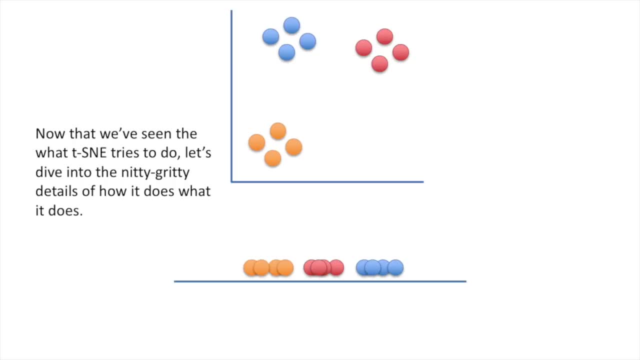 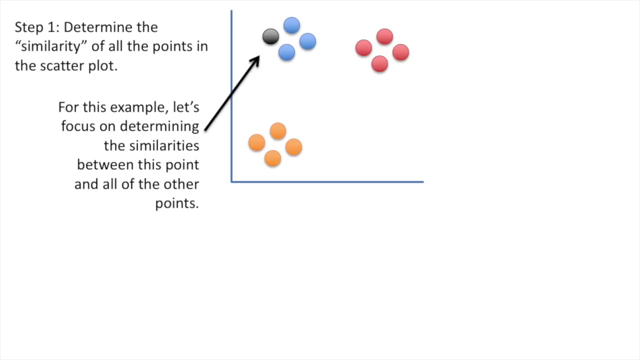 Now that we've seen what t-SNE tries to do, let's dive into the nitty-gritty details of how it does what it does. Step 1. Determine the similarity of all the points in the scatter plot. For this example, let's focus on determining the similarities between this point and all. 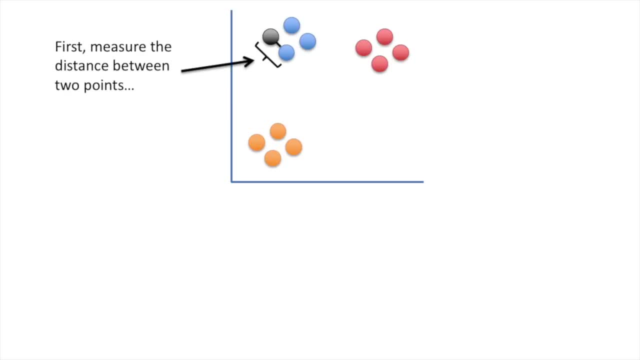 of the other points. First measure the distance between two points. Then plot that distance on a normal curve that is centered on the point of interest. Lastly, draw a line from the point to the curve. The length of that line is the unscaled similarity. 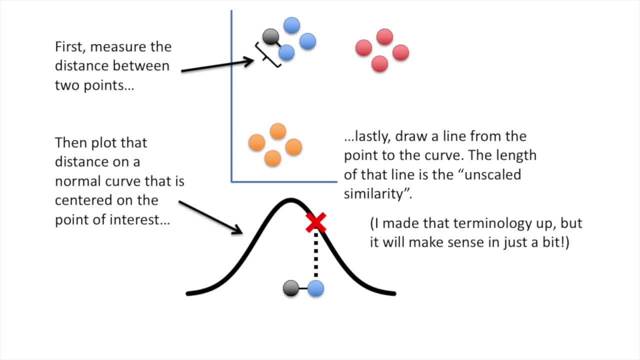 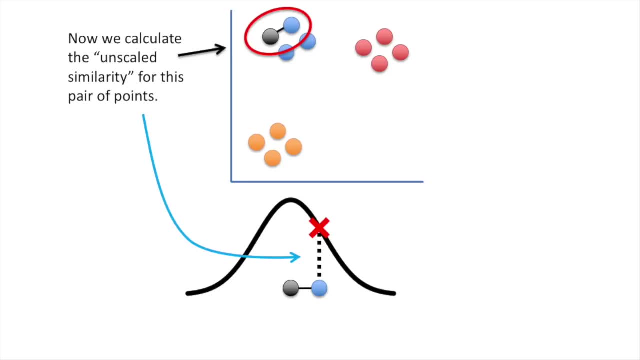 I made that terminology up, but it'll make sense in just a bit, so hold on. Now we calculate the unscaled similarity For this pair of points. Now we calculate the unscaled similarity For this pair of points. And now we calculate the unscaled similarity. 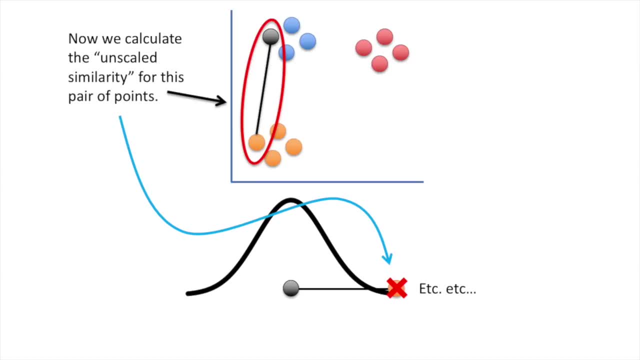 For this pair of points, Etc. etc. etc. Using a normal distribution means that distant points have very low similarity values And close points have high similarity values. Ultimately, We measure the distances between all of the points and the point of interest. 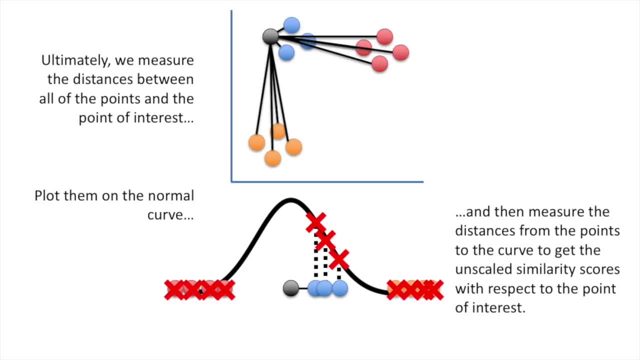 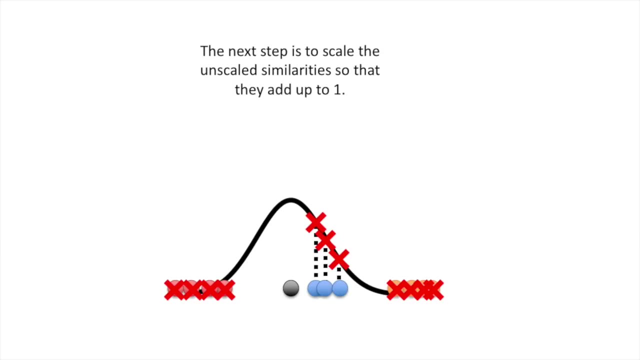 Then plot them on a normal curve And then measure the distances from the points to the curve to get the unscaled similarity scores with respect to the point of interest. The next step is to scale the unscaled similarities so that they add up to 1.. 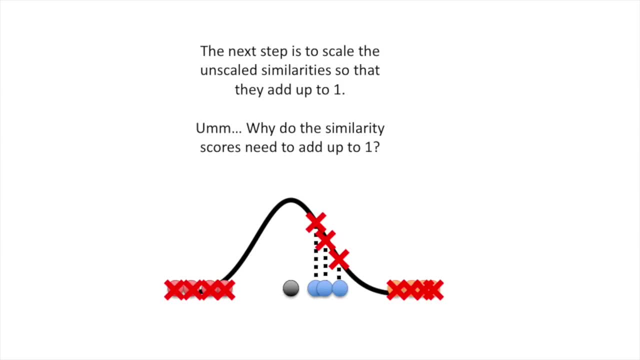 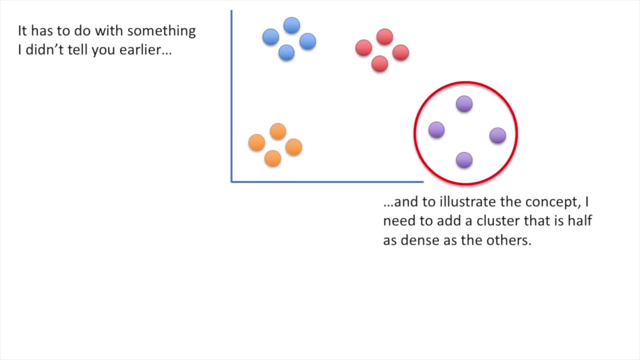 Ummm, Why do the similarity scores need to add up to 1?? I don't know. It has to do with something I didn't tell you earlier, And to illustrate the concept, I need to add a cluster that is half as dense as the others. 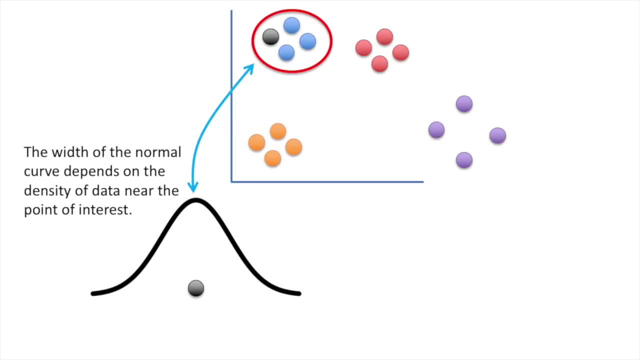 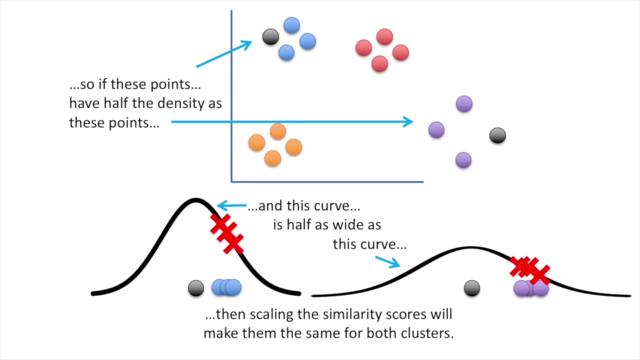 The width of the normal curve depends on the density of data near the point of interest. Less dense regions have wider curves. So if these points have half the density as these points and this curve is half as wide as this curve, Then scaling the similarity scores will make them the same for both clusters. 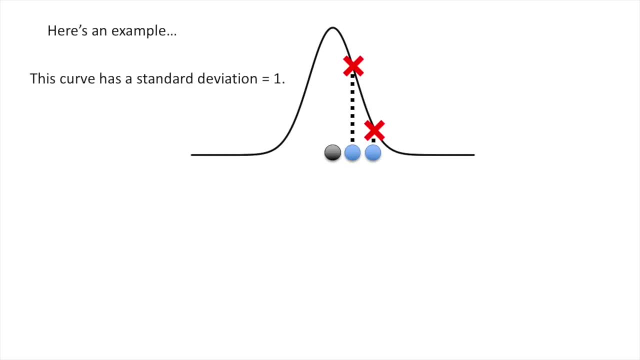 Here's an example where I've worked out the math. This curve has a standard deviation equal to 1.. These are the unscaled similarity values. This curve has a standard deviation equal to 2.. These points are twice as far from the middle. 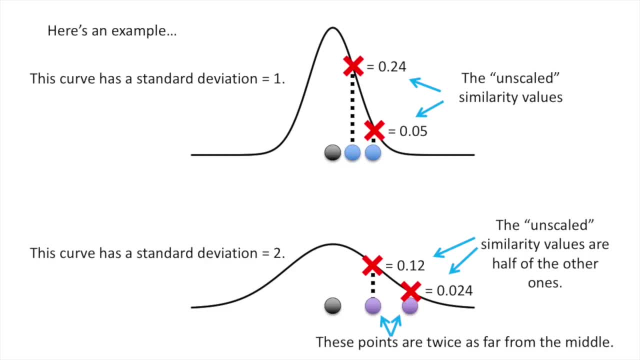 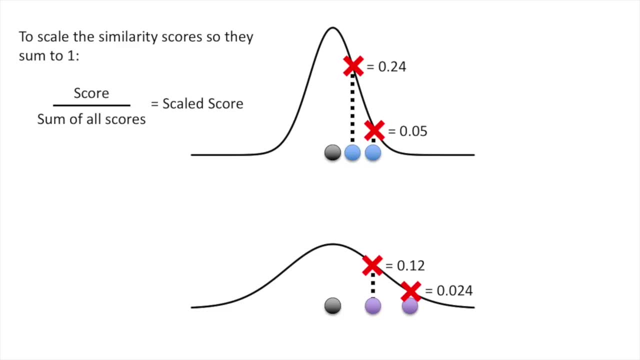 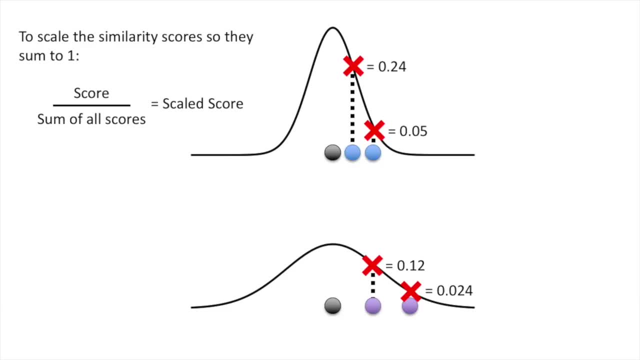 it by the sum of all the scores. That equals the scaled score. Here's how the math works out when the distribution has a standard deviation equal to 1. We get 0.82 and 0.18 as the scaled similarity scores. 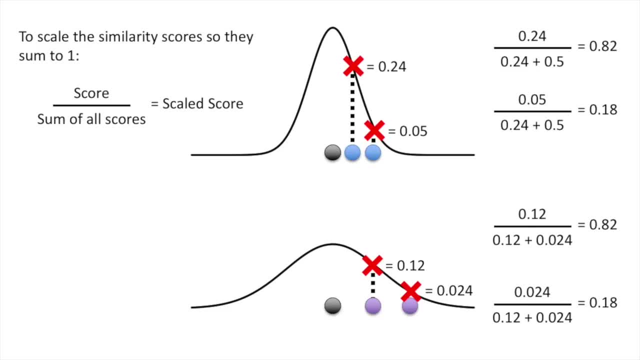 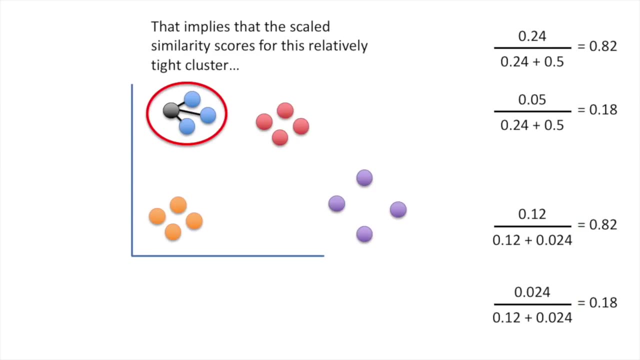 And here's the math for when everything is spread. When everything is spread out twice as much, we get 0.82 and 0.18.. The similarity scores on top are equal to the similarity scores below. They're the same. That implies that the scaled similarity scores for this relatively tight cluster are the 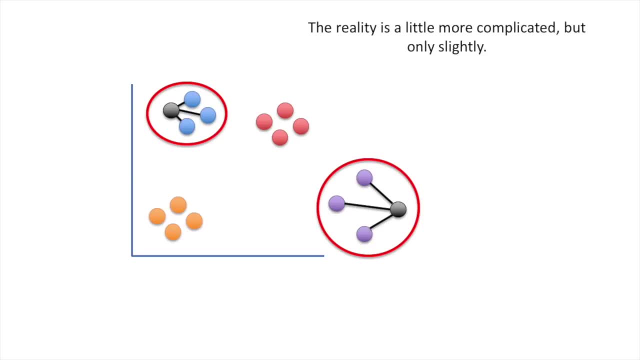 same for this relatively loose cluster. The reality is a little more complicated, but only slightly. T-SNE has a perplexity parameter equal to the expected density around each point And that comes into play. But these clusters are still more similar than you might expect. 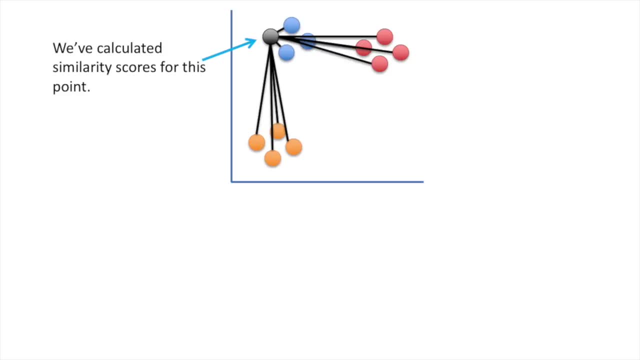 Now back to the original scatter plot. We've calculated similarity scores for this point. Now we do it for this point And we do it for all the points. One last thing: The scatter plot will be all set with similarity scores, Because the width of the distribution is based on the density of the surrounding data points. 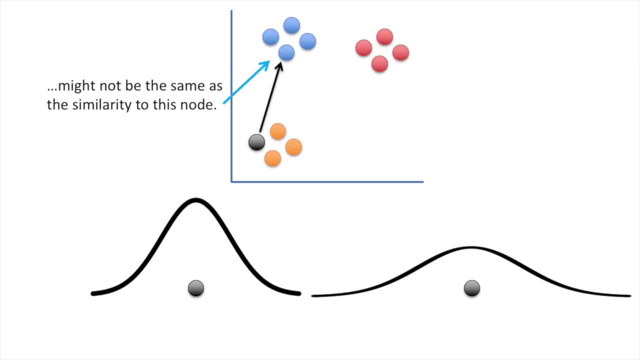 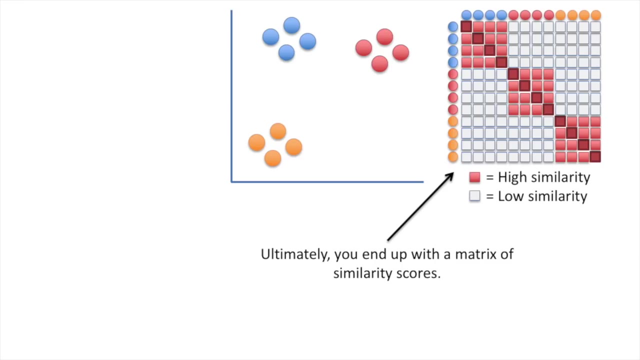 the similarity score for this node might not be the same as the similarity to this node, So T-SNE just averages the two similarity scores from the two directions. No big deal. Ultimately you end up with a matrix of similarity scores. Each row and column represents the similarity scores calculated from that point of interest. 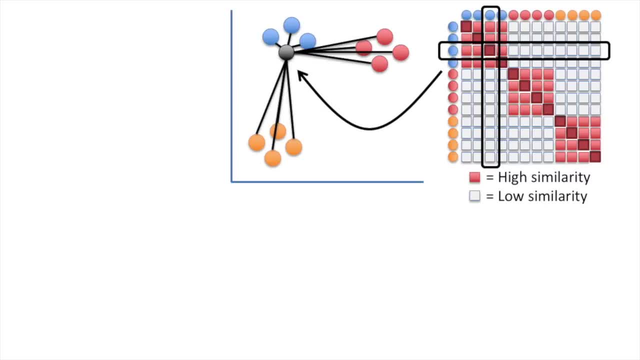 Red equals high similarity and white equals low similarity. I've drawn the similarity from a point of interest to itself as dark red. However, it doesn't really make sense to say that a point is similar to itself, because that doesn't help the clustering. 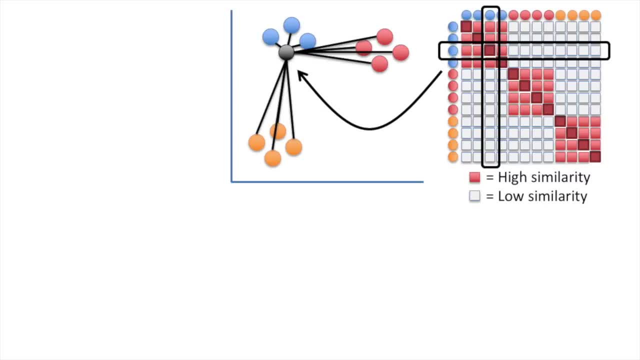 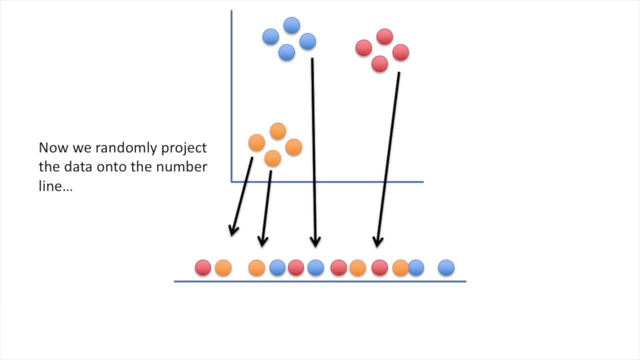 So T-SNE actually defines that similarity as zero. Hooray, We're done calculating similarity scores for the scatter plot. Now we randomly project the data onto the number line and calculate similarity scores for the points on the number line, Just like before. that means picking a point. 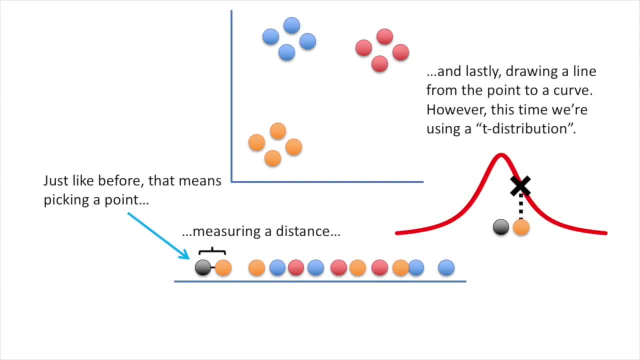 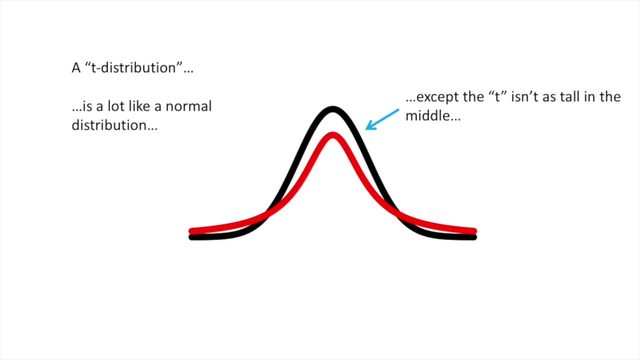 measuring a distance and, lastly, drawing a line from the point to a curve. However, this time we're using a T-distribution. A T-distribution is a lot like a normal distribution, except the T isn't as tall in the middle. 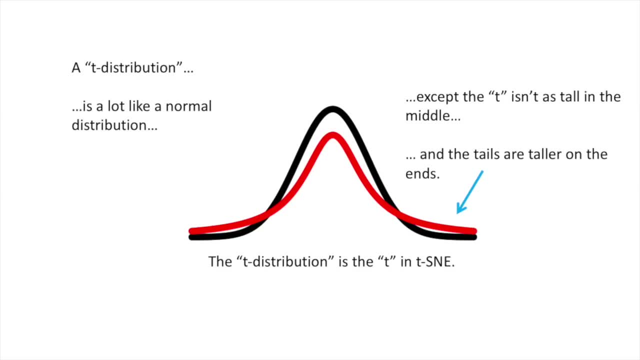 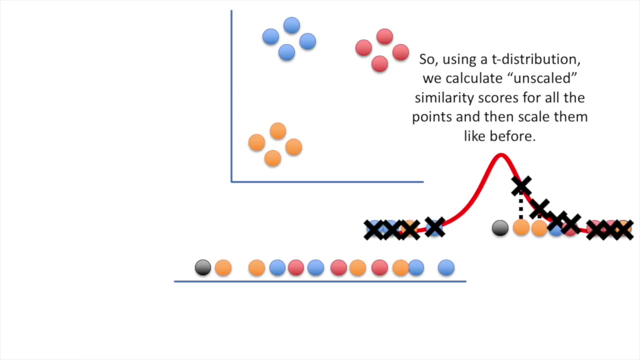 and the tails are taller on the ends. The T-distribution is the T in T-SNE. We'll talk about why the T-distribution is used in a little bit. So using a T-distribution, we calculate unscaled similarity scores for all the points. 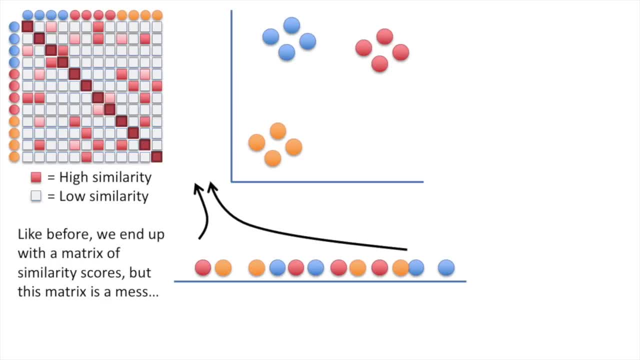 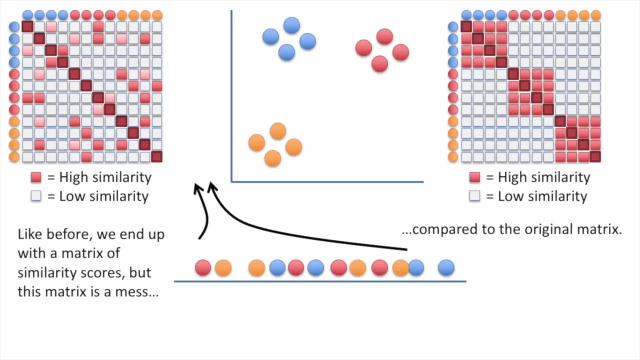 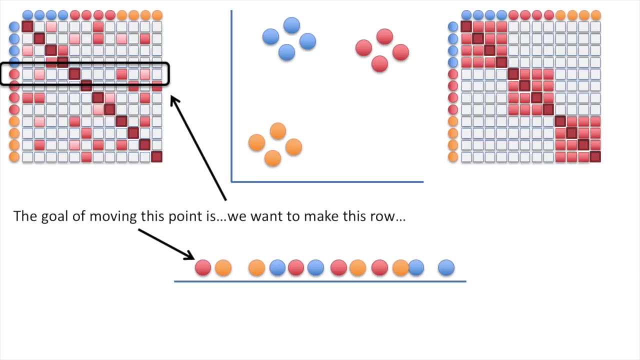 and then scale them like before. Like before, we end up with a matrix of similarity scores. but this matrix is a mess compared to the original matrix. The goal of moving this point is: we want to make this row look like this row. 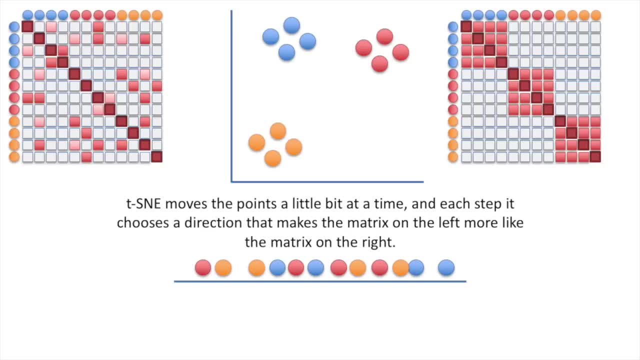 T-SNE moves the points a little bit at a time and at each step it chooses a direction that makes the matrix on the left more like the matrix on the right. It uses small steps because it's a little bit like a chess game. 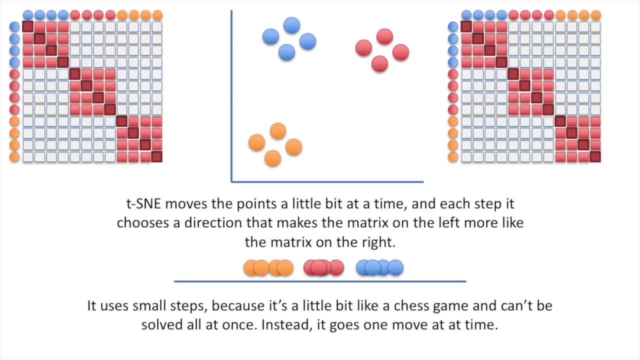 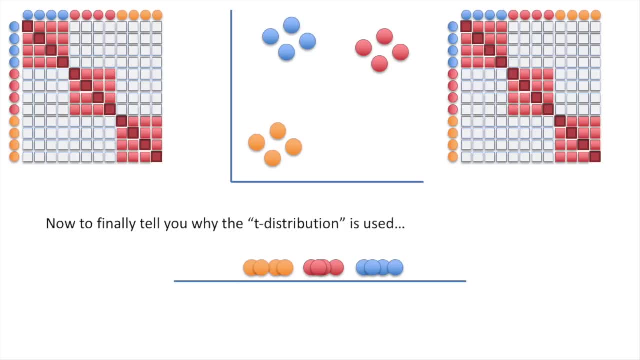 and can't be solved all at once. Instead, it goes one move at a time. BAM Now to finally tell you why the T-distribution is used. Without it, the clusters would all clump up in the middle and be harder to see.